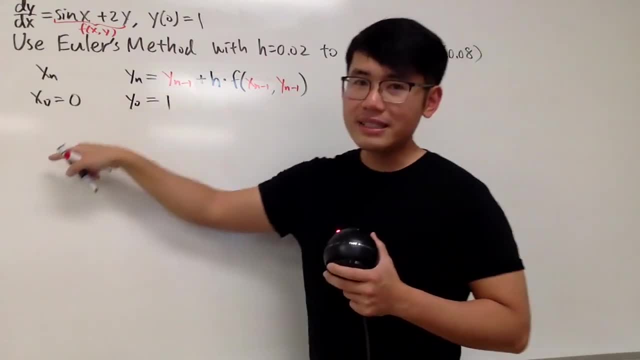 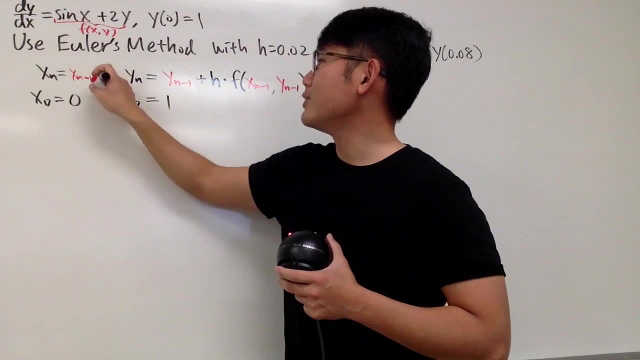 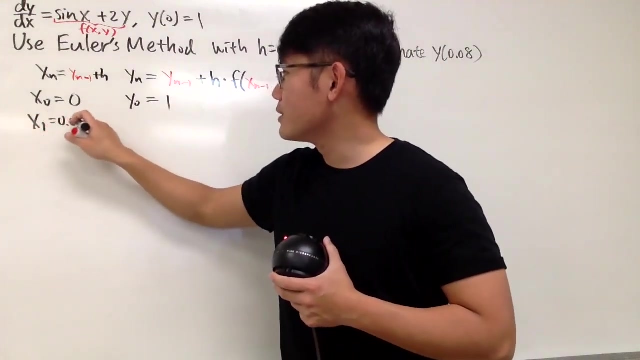 So that's our starting, And now to get the next x value, you just go ahead and just technically you should do xn-1 plus h, So you just pretty much keep adding 0.02.. So the next one is x1,, which is 0.02, like that. 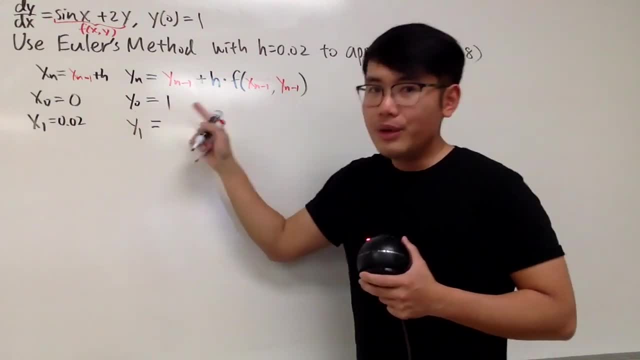 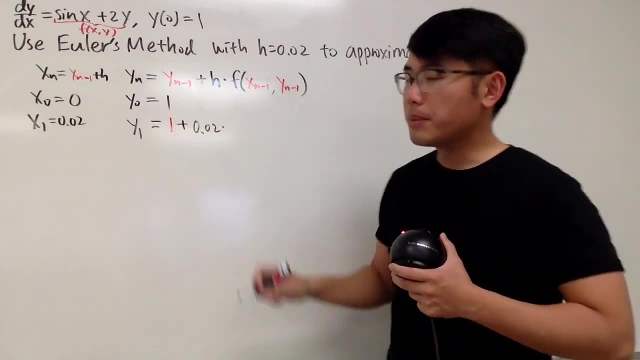 Alright, y1,. this, right here You are going to look at the previous y value, which is 1, and then you add: h is 0.02, and then you multiply by f of the previous x and y value. right, 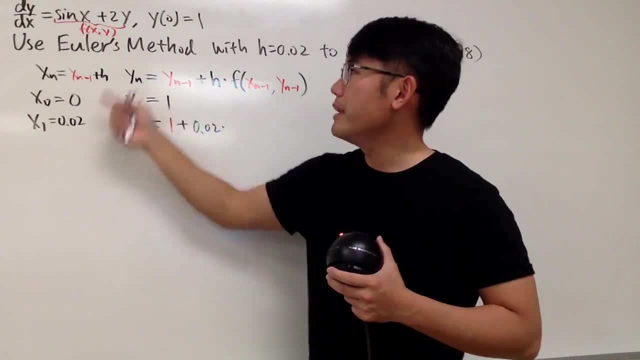 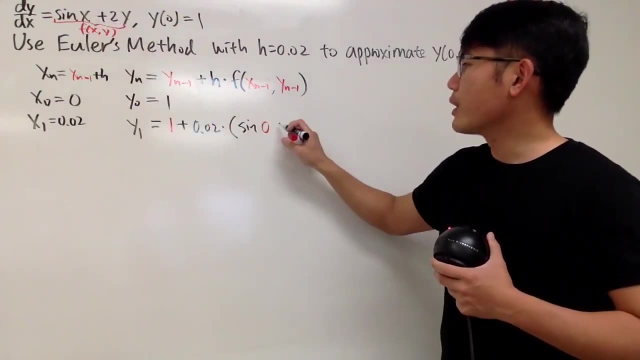 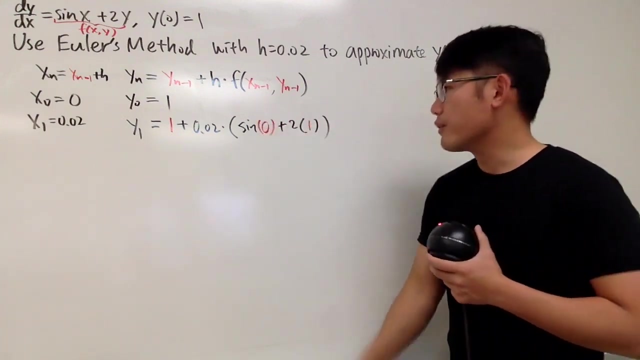 So you are going to look at the previous x and y value, Put them into here. So I'll just put a parenthesis: You put 0 into sin and then you are going to add 2 times 1, like that. So that's pretty much the idea, And, of course, just use a calculator if you like. This is not that bad at all. 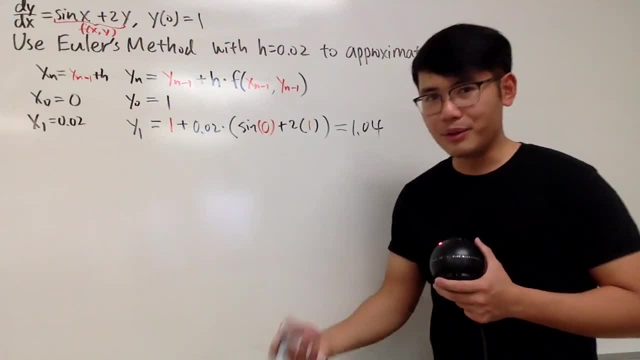 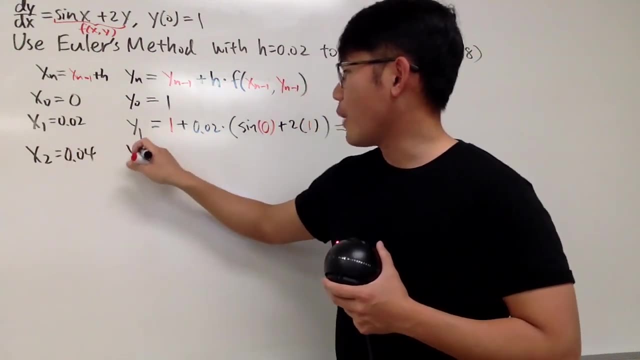 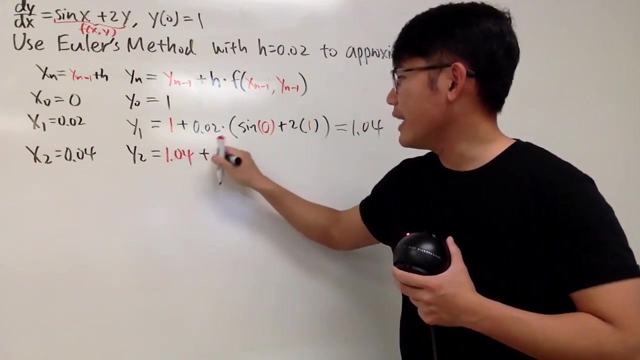 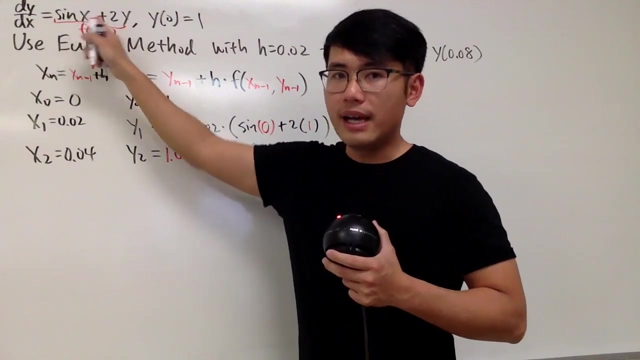 You get 1.04, and now you pretty much just continue the process. Next one, x2,. you just keep adding the h, right? So you get 0.04, and then y2.. So this is going to be the previous y value, which is 1.04, and then we add the h value, which is 0.02, and then we're throwing this and that into the f, which is the x and y, right there. 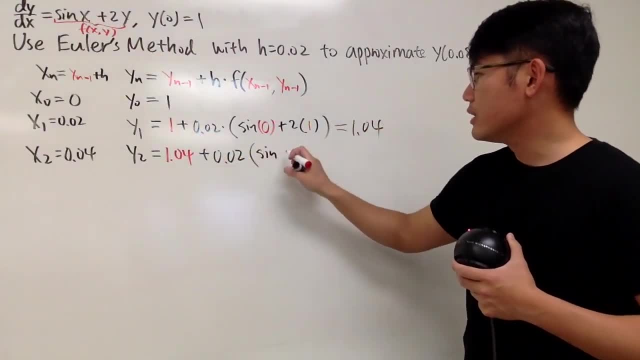 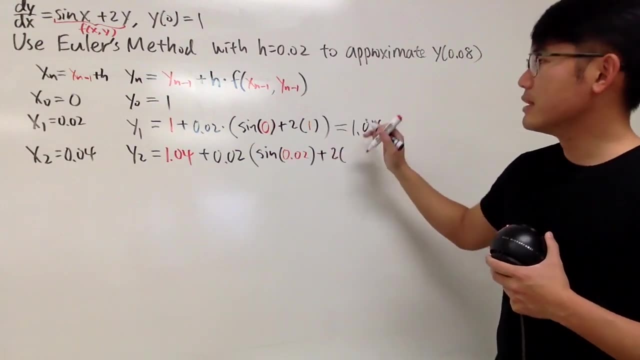 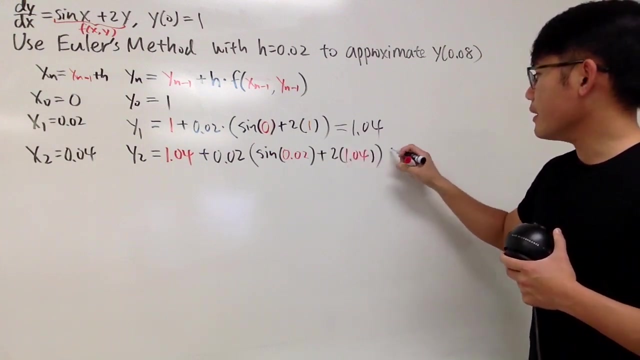 So we get sin of 0.02, and then we are going to add 2 times this, because you put this into the y over there, so 1.04.. And now, if you do that, you will end up with 1.0820.. 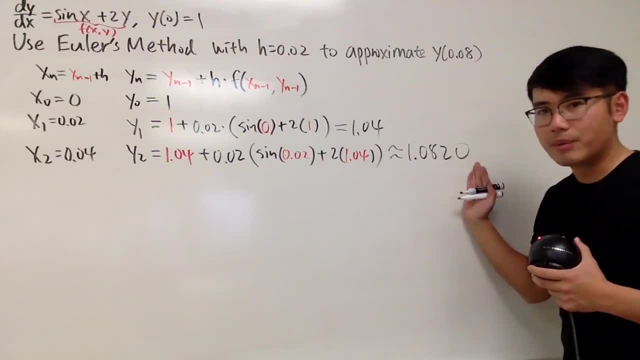 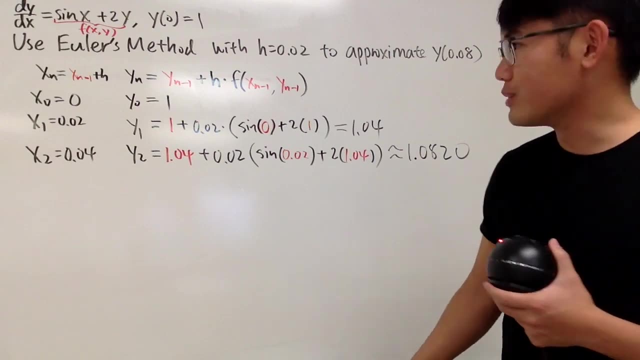 So I'm just doing this up to the fourth decimal place, right here, right? So I'm looking at the numbers, of course, And then I will just continue. x3, this is equal to 0.06.. And then you just go ahead. 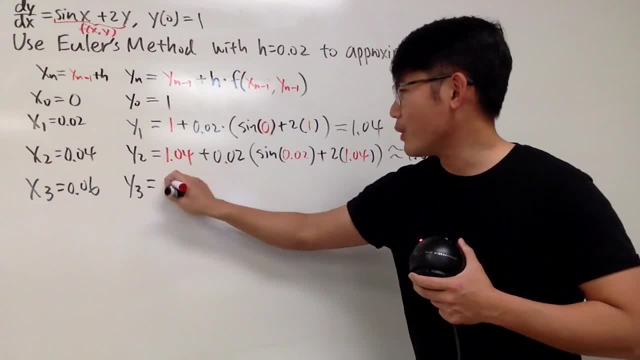 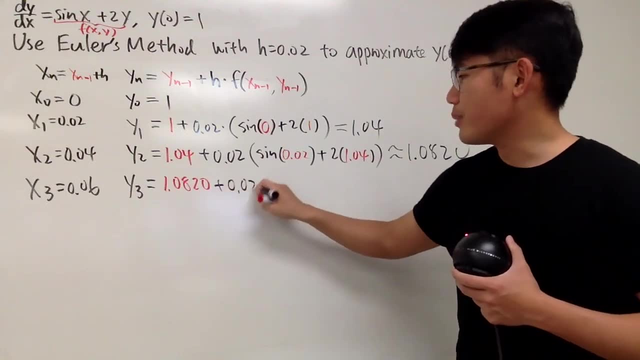 y3 is equal to the previous y value, which is 1.0820.. Well, just the 0 doesn't matter, you know that. And then, plus again, h is 0.02.. h doesn't change throughout the whole process. 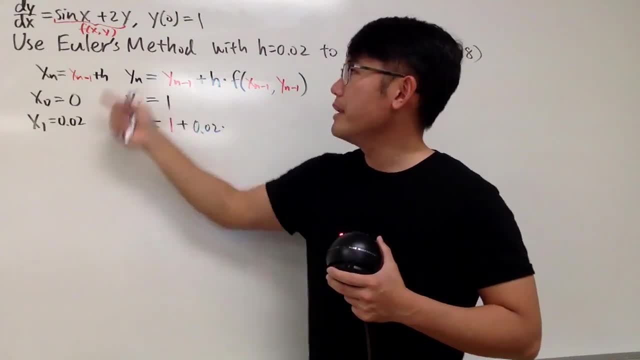 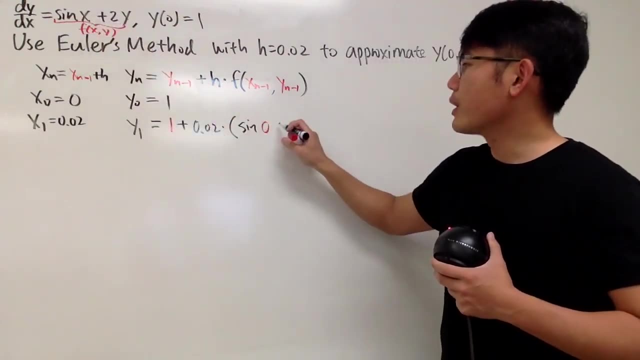 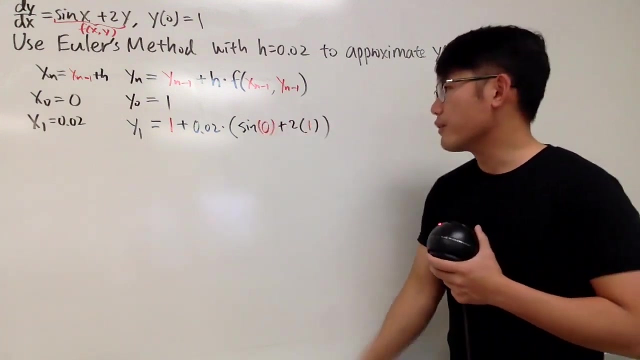 So you are going to look at the previous x and y value, Put them into here. So I'll just put a parenthesis: You put 0 into sin and then you are going to add 2 times 1, like that. So that's pretty much the idea, And, of course, just use a calculator if you like. This is not that bad at all. 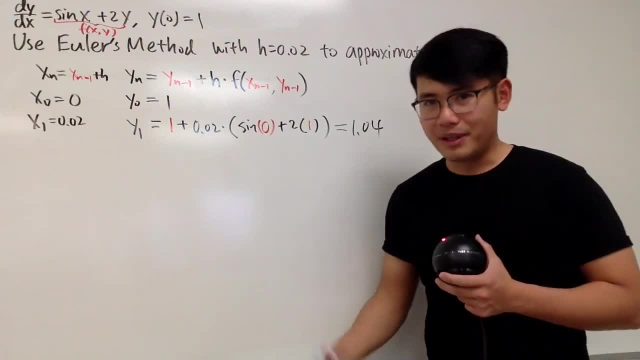 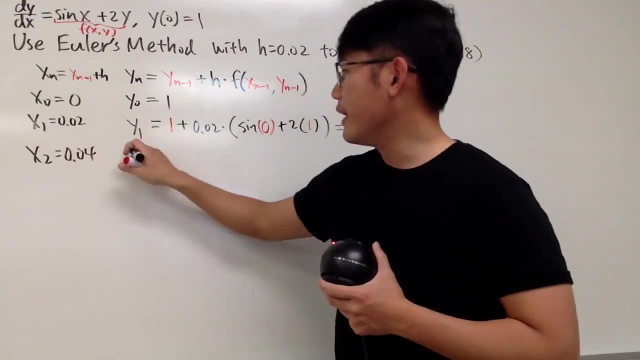 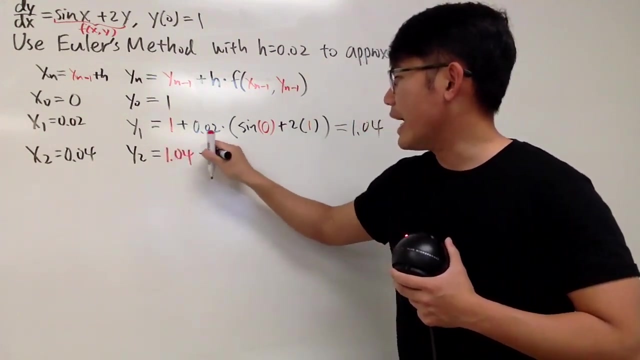 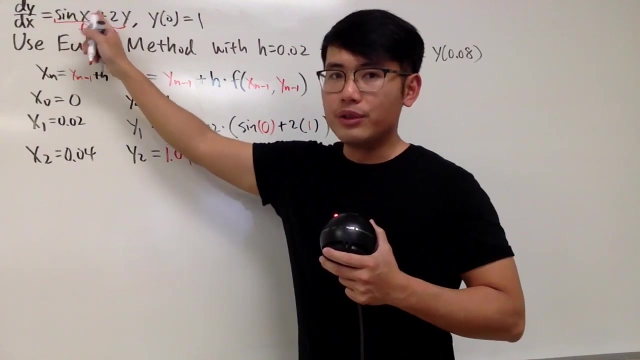 You get 1.04.. And now you pretty much just continue the process. Next one: x2,. you just keep adding the h, right? So you get 0.04, and then y2.. So this is going to be the previous y value, which is 1.04, and then we add the h value, which is 0.02, and then we're throwing this and that into the f, which is the x and y, right there. 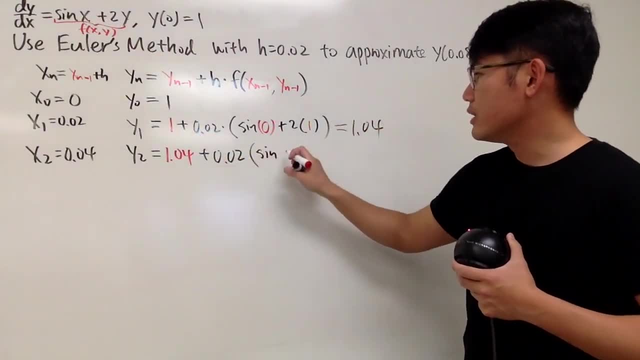 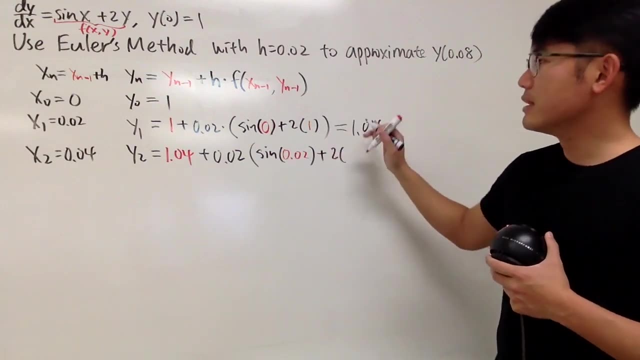 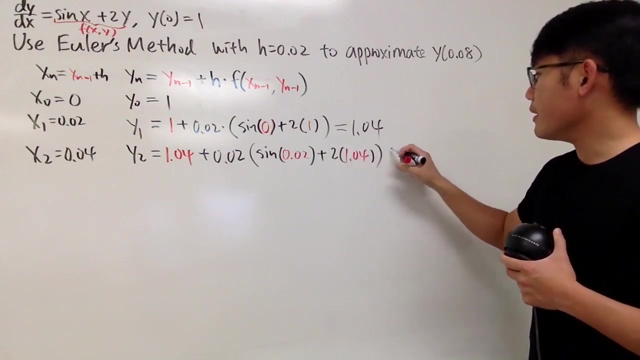 So we get sin of 0.02, and then we are going to add 2 times this, because you put this into the y over there, so 1.04.. And now, if you do that, you end up with 1.0820.. 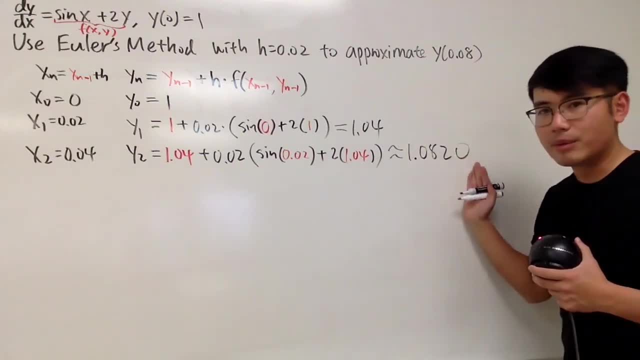 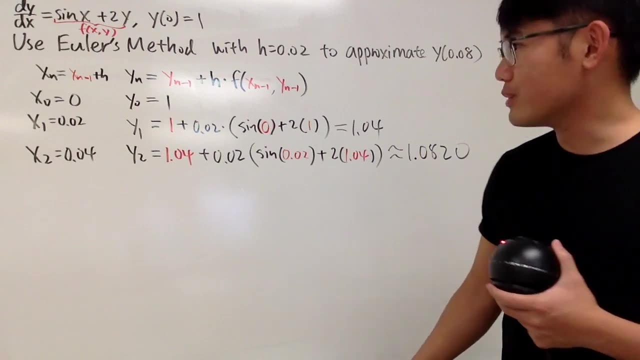 So I'm just doing this up to the 4th decimal place, right here, right? So I'm looking at the numbers, of course, And then I will just continue. x3, this is equal to 0.06.. And then you just go ahead. 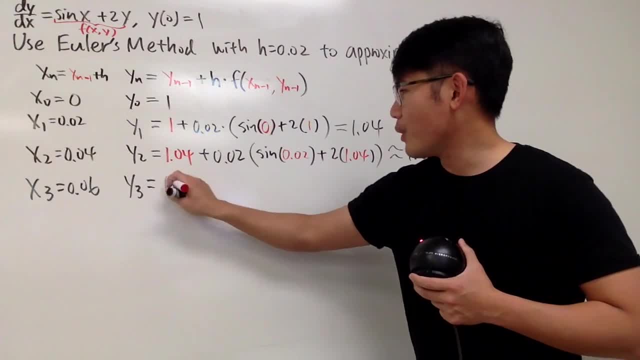 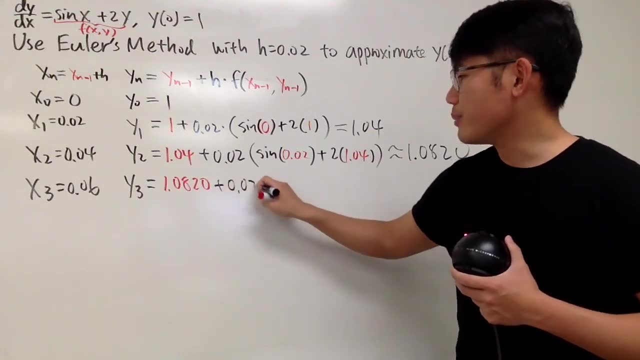 y3 is equal to the previous y value, which is 1.0820,. well, just the 0 doesn't matter, you know that. And then, plus again, h is 0.02,. h doesn't change throughout the whole process. 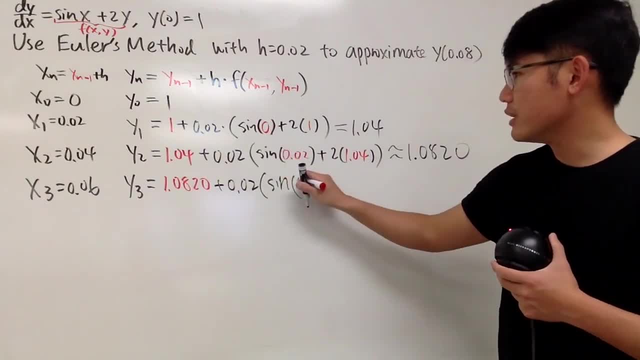 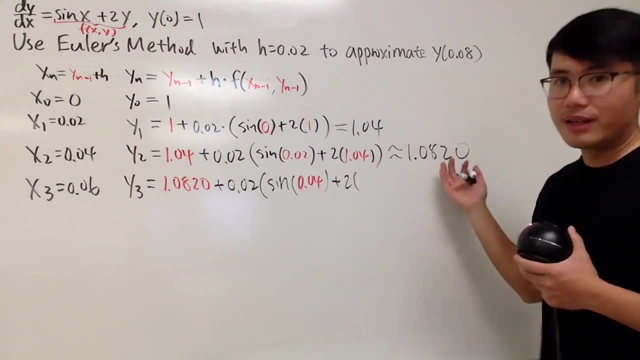 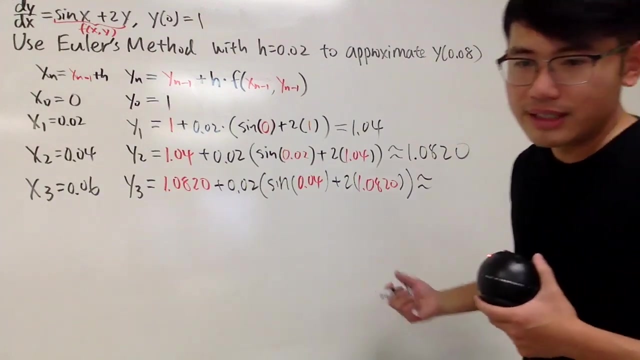 and then sine of the previous x value, which is 0.04, and then we add 2 times the previous y value, 1.0820,, like this. And again, I challenge you guys, if you guys, you can just do this in your head, but I cannot. 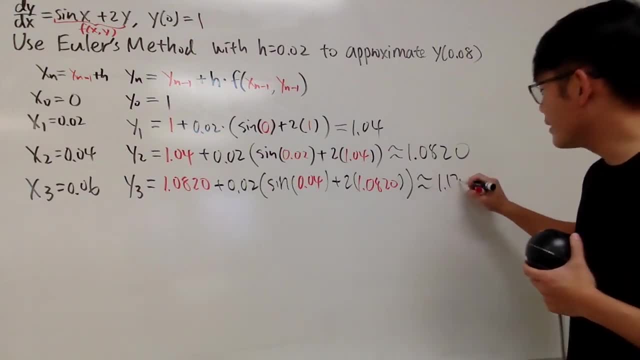 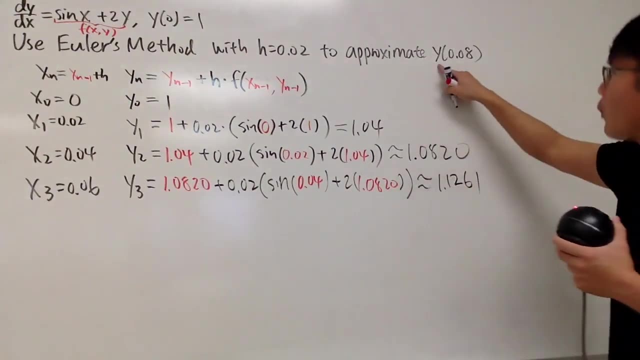 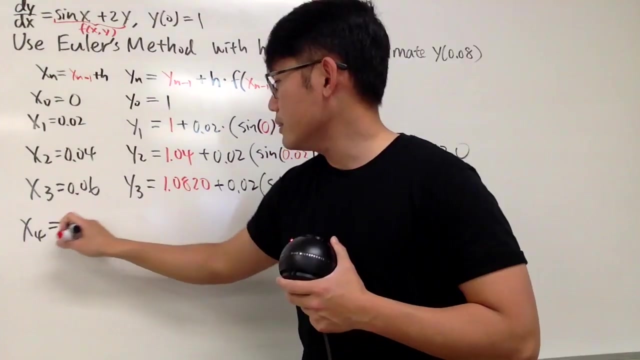 I'll use a calculator. we'll just look at the answer that I already prepared: 1.1261, right, One more, because you see we want to end up y of 0.08.. So the x value for this one is going to be precisely equal 0.08,. 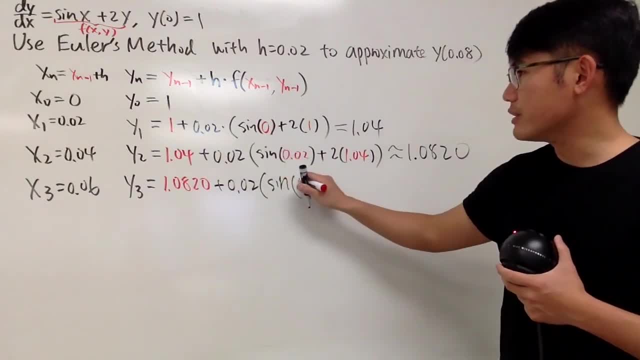 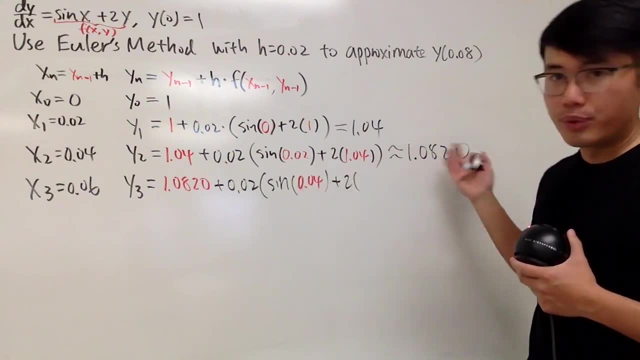 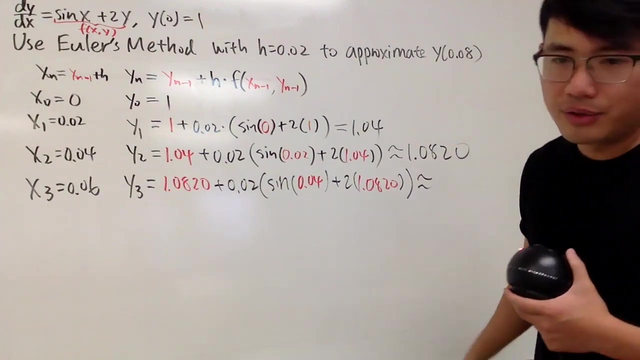 And then sin of the previous x value, which is 0.04.. And then we add 2 times the previous y value, 1.0820, like this. And again, I challenge you, if you guess you can just do this in your head. 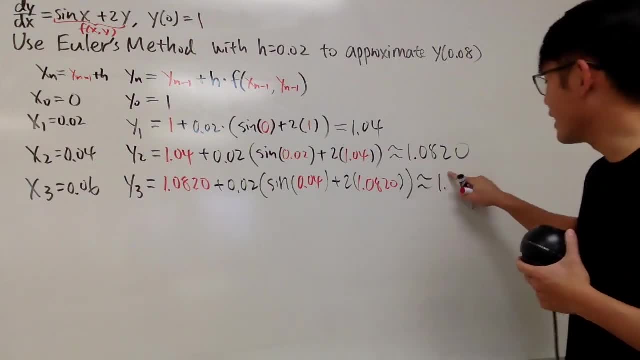 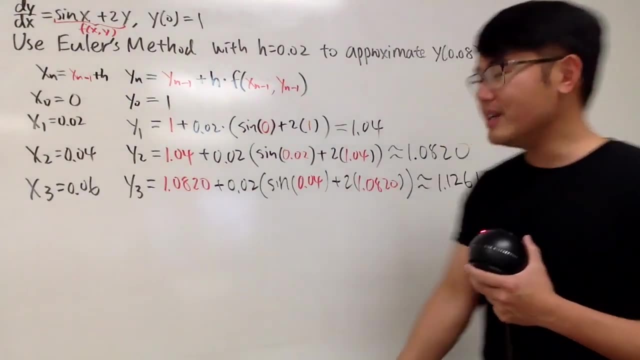 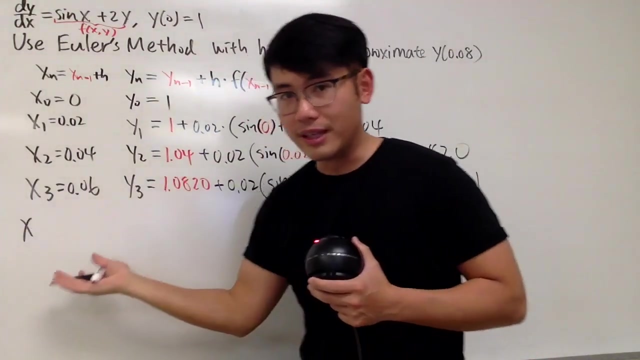 But I cannot, I will use a calculator. We'll just look at the answer that I already prepared: 1.1261.. Right, One more, Because you see we want to end up y of 0.08.. So the x value for this one is going to be precisely equal 0.08.. 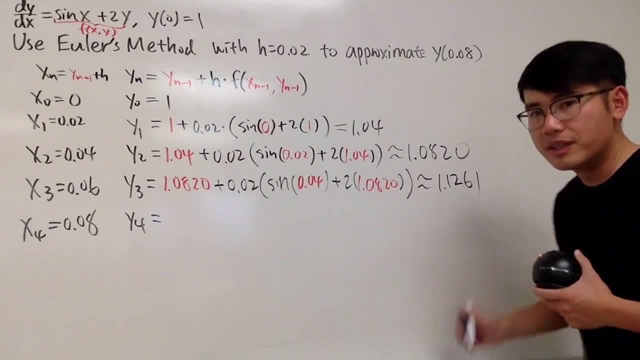 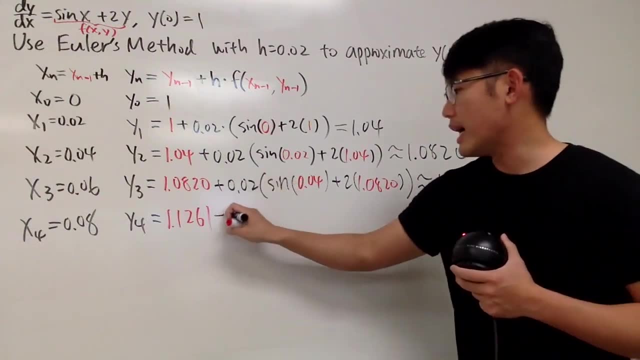 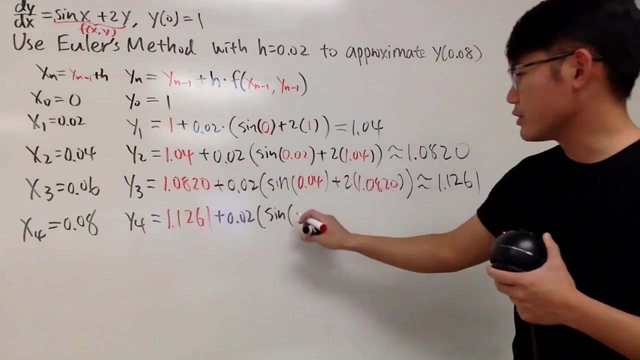 And then y4, again put down the previous y value, which is 1.1261.. And then, Again, you add the h, which is 0.02, and then times sin of the previous x value, which is that. 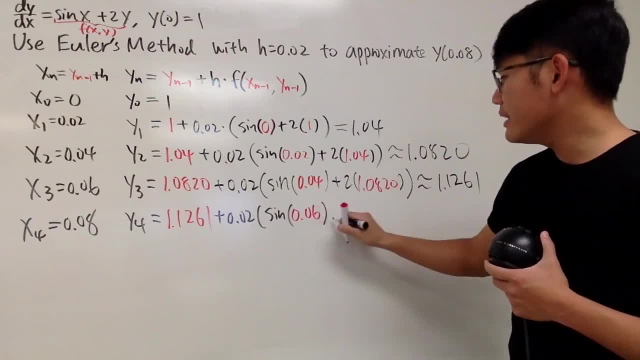 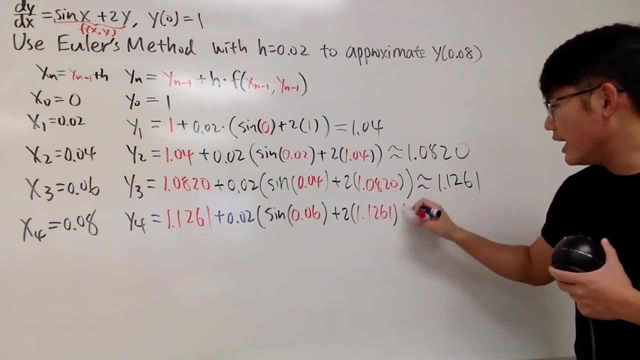 So just put in there 0.06.. And then you add 2 times the previous y value, which is 1.1261,. like this Right, And in the end you will get approximately 1.1723. Right. 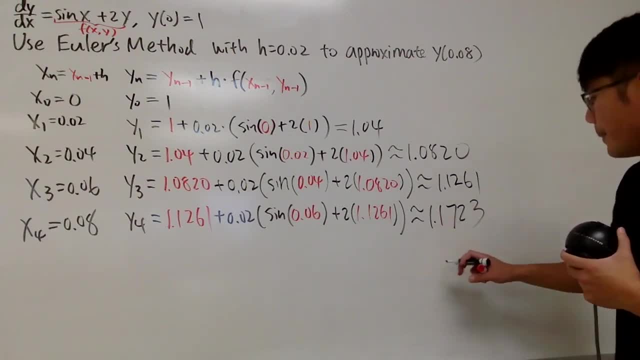 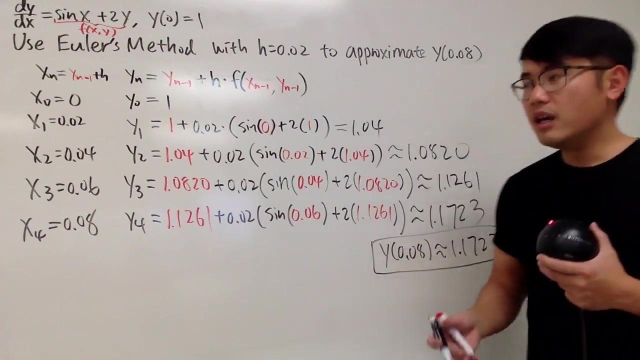 I'm just using these four decimal places for it. So based on this, we are saying y of 0.08 is approximately 1.1723.. So this right here will be the approximation based on the Euler's method And of course I know a lot of you guys would like to know how to solve this differential equation from scratch. 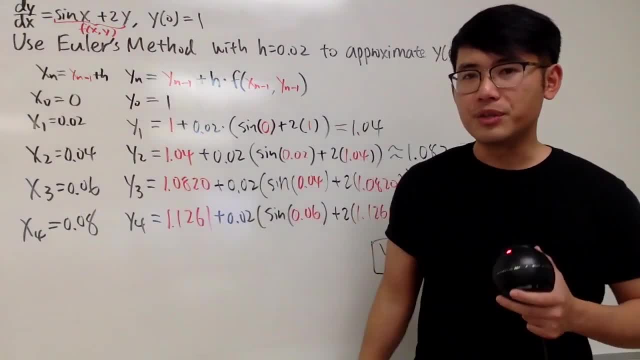 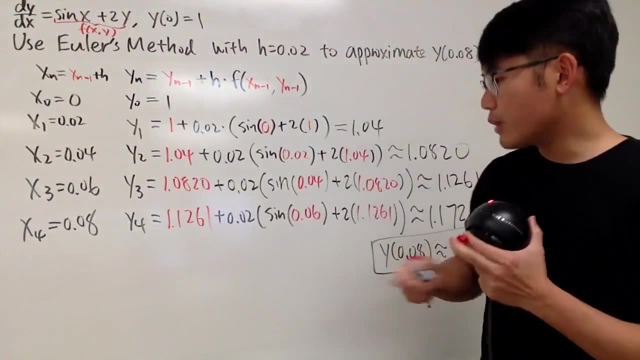 I have the video already for you guys, so be sure you guys check the link in the description if you haven't seen that already. And of course, let's compare the values right here, Right? So I'll write that down for you guys. 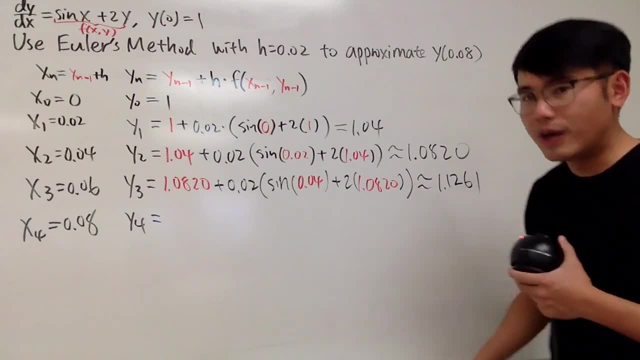 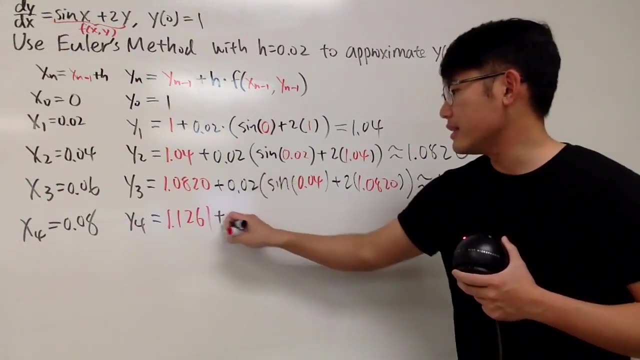 and then y4, again put down the previous y value, which is 1.0820,, 1.1261, and then again you add the h, which is 0.02, and then times sine of the previous x value, which is that. 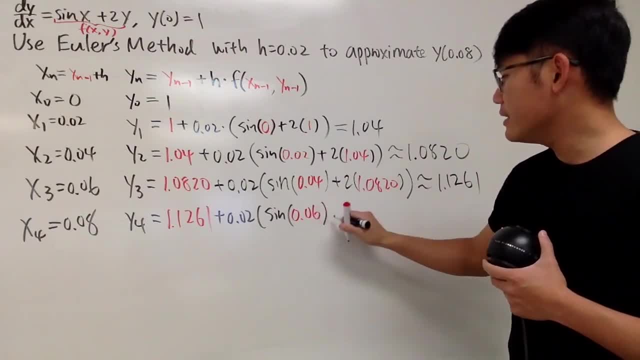 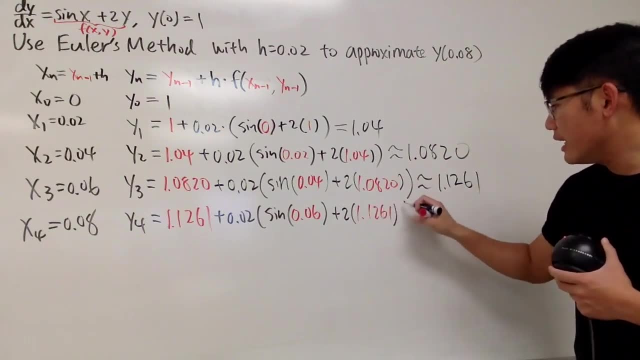 so just put in there 0.06, and then you add 2 times the previous y value, which is 1.1261,. like this right, And in the end you will get approximately 1.1723, right. 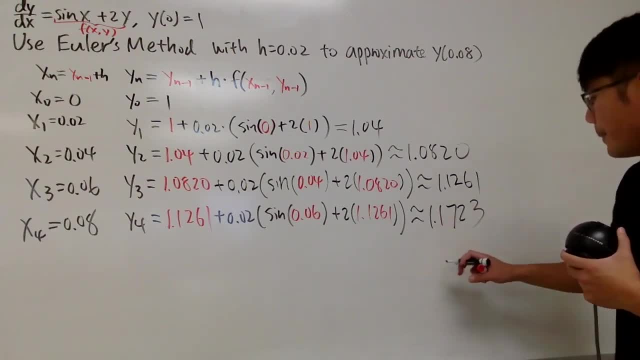 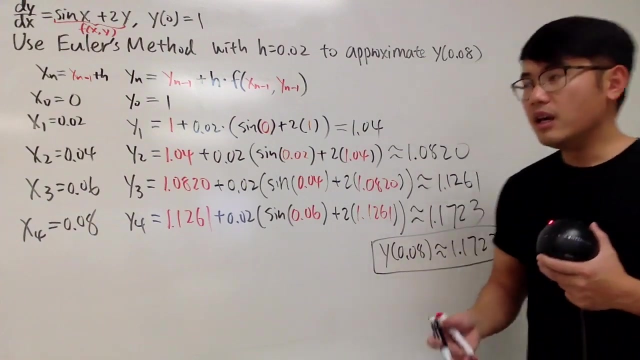 I'm just using this: 4. There's more places for it. So based on this, we are saying y of 0.08 is approximately 1.1723.. So this right here will be the approximation based on the Euler's method. 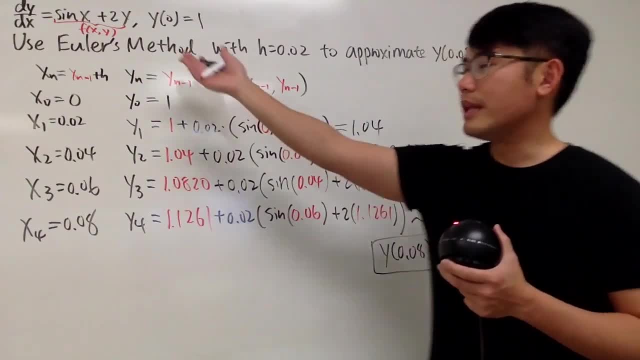 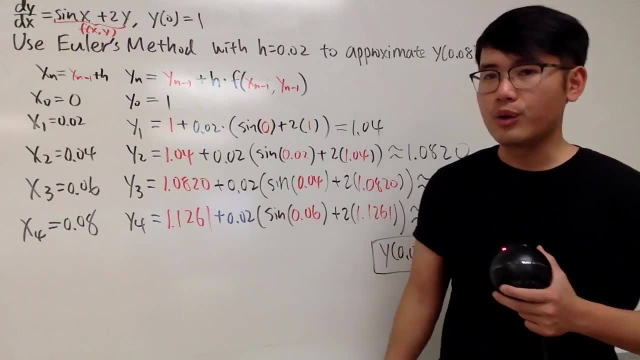 And of course I know a lot of you guys would like to know how to solve this differential equation from scratch. I have the video already for you guys. so be sure you guys check the link in the description if you haven't seen that already. 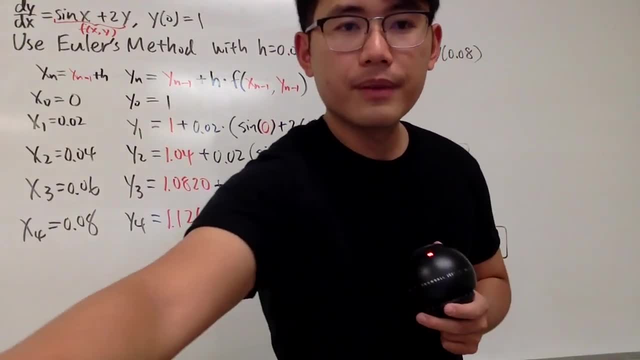 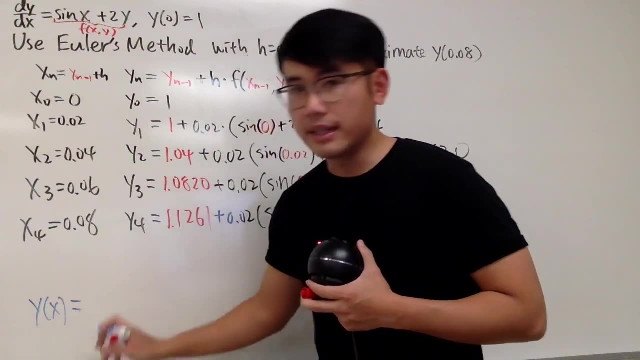 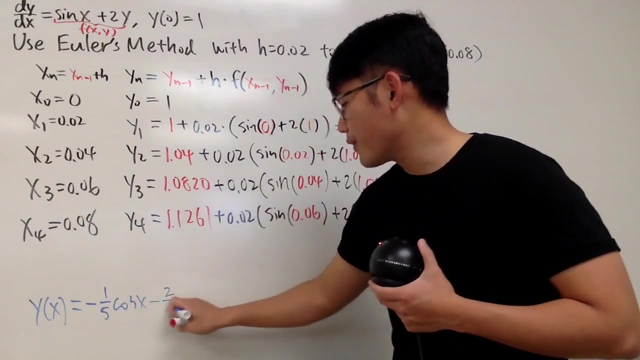 And of course, let's compare the values Right here, right? So I'll write that down for you guys. The truth is y of x. y as the function of x. this is equal to negative 1 over 5 cosine x, minus 2 over 5 sine x. 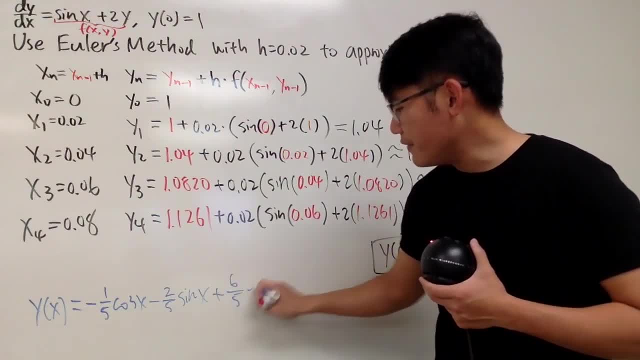 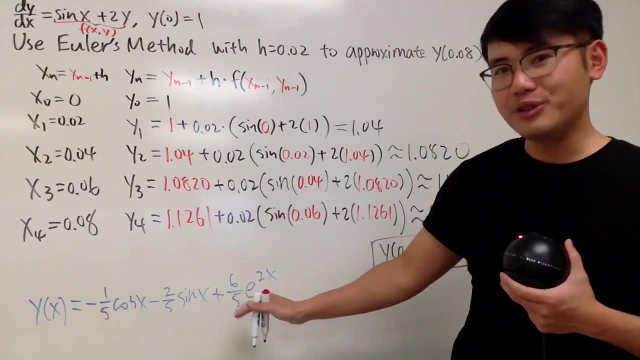 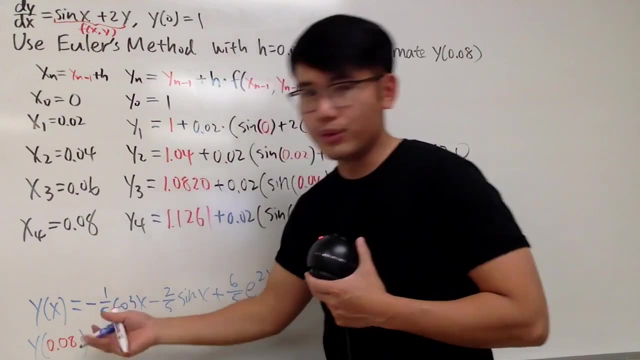 and then, lastly, we have plus 6 over 5 e to the 2x. And then, if you put in 0.08 into all the x by using the actual solution, let me tell you: y of 0.08, again, just let x equal to this 0.08,. 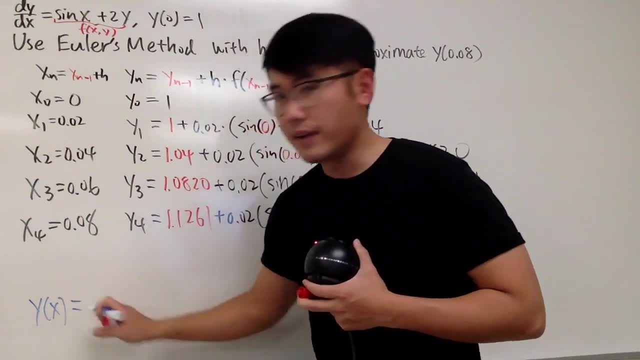 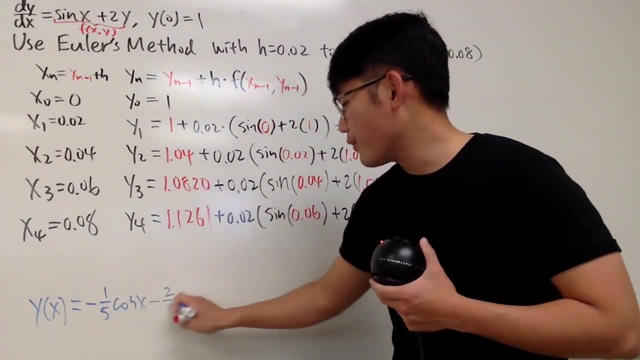 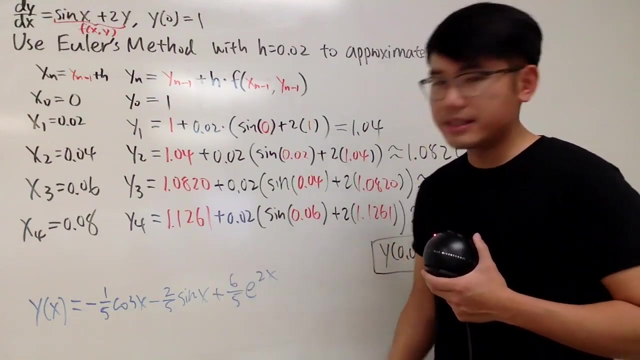 The truth is y of x, y as a function of x. this is equal to negative 1 over 5 cosine x, minus 2 over 5 sine x. And then, lastly, we have plus 6 over 5, e to the 2x. 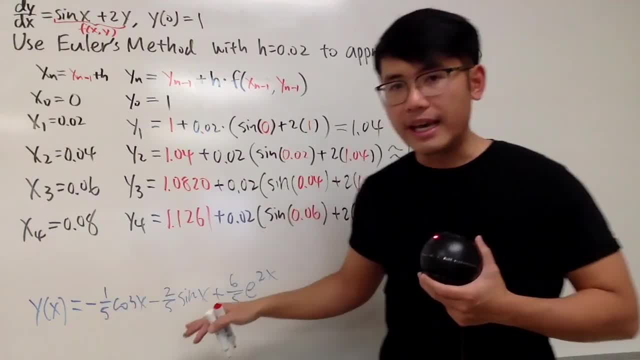 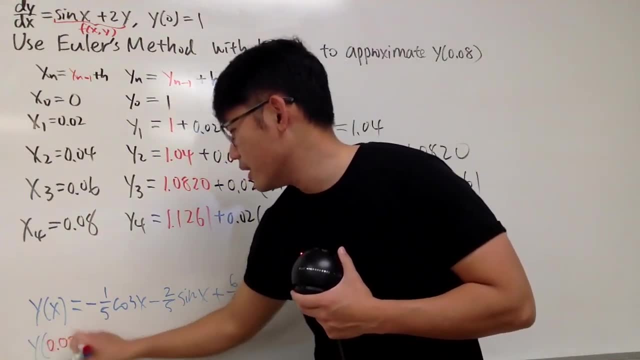 And then if you put in 0.08 into all the x by using the actual solution, let me tell you: y of 0.08.. 0.08.. Again, just that x equal to this 0.08.. 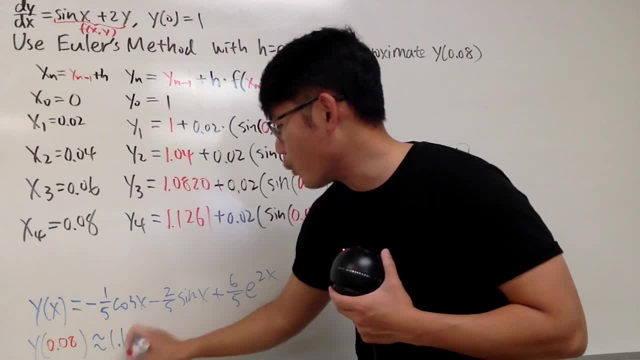 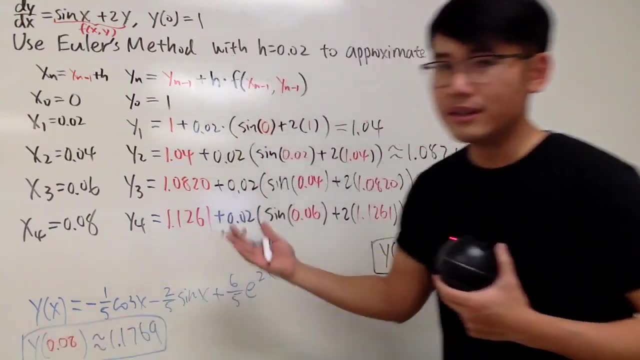 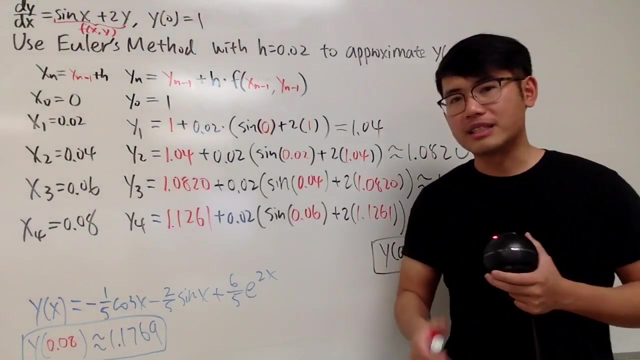 and you'll actually end up with 1.1769 approximately speaking right. So this is the actual solution and this is our approximation. As you can see, it's actually pretty close, right? That's it. Leave a comment down below and let me know if you guys have any questions. 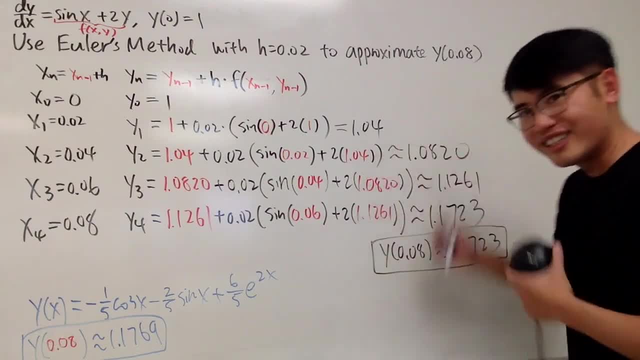 If you guys are new to my channel, be sure to subscribe. Thank you guys. so much and, as always, that's it. 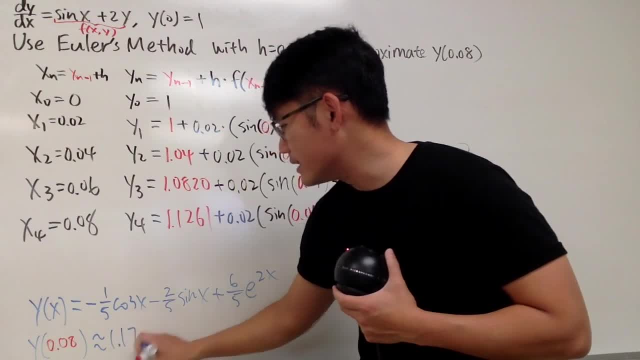 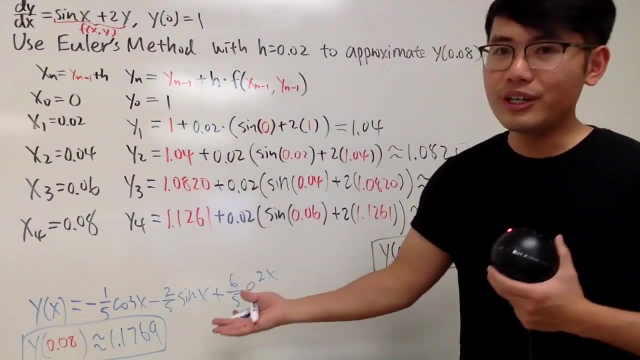 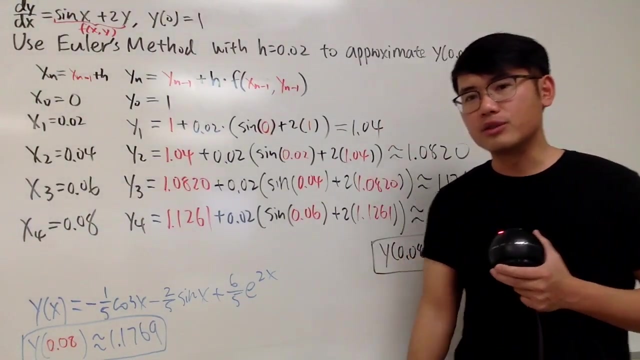 And you actually end up with 1.1769 approximately speaking Right. So this is the actual solution And this is our approximation. As you can see, it's actually pretty close, Right? That's it. Leave a comment down below and let me know if you guys have any questions. If you guys are new to my channel, be sure to subscribe. Thank you guys so much And, as always, that's it. 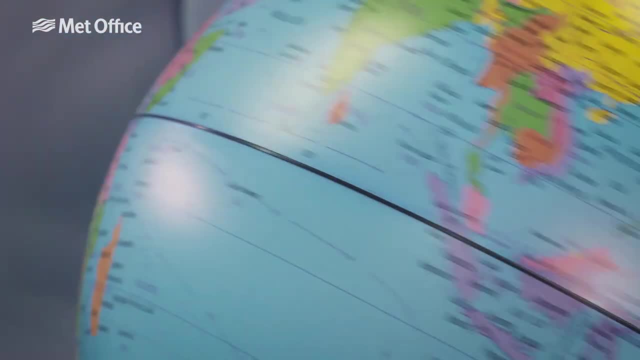 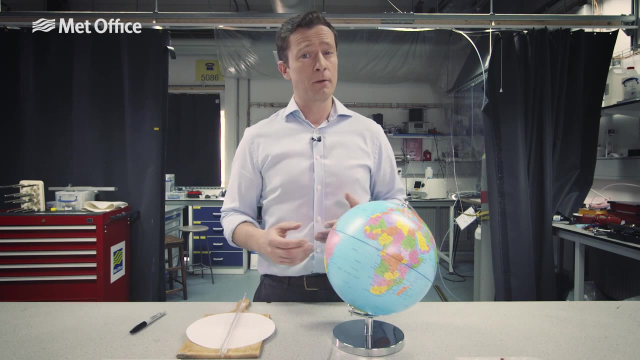 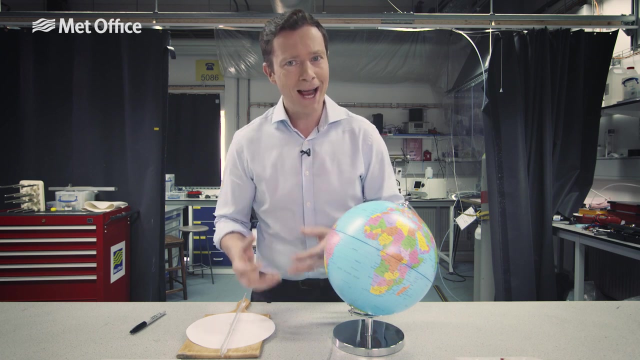 Okay, so we know the earth is spinning on its axis and this spin has implications for the direction of the wind. We call this Coriolis. Now you may have heard of the Coriolis effect or the Coriolis force, but this is not a real force. It's what we call an apparent force. It all depends on your. 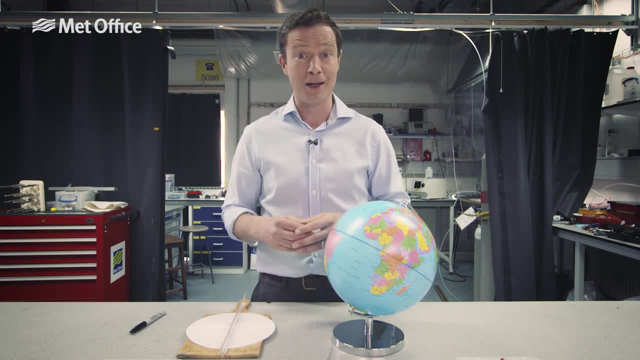 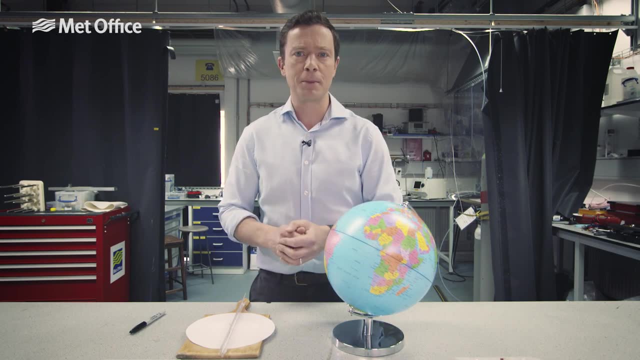 point of view, whether you're looking down from above or, like most of us, are on the earth, looking from below upwards. Now, this is quite a complicated sounding business, but I've got a simple experiment to show it here: Chopping board. we've got a disc of paper pinned to that chopping board. 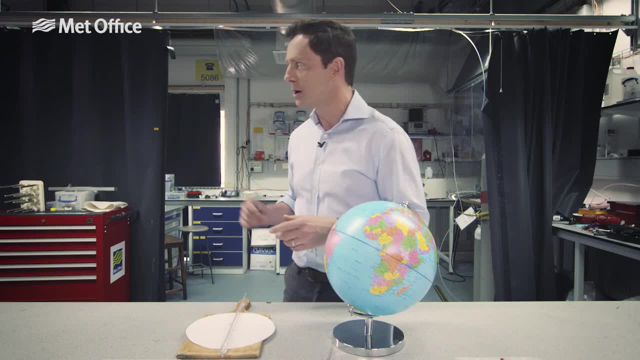 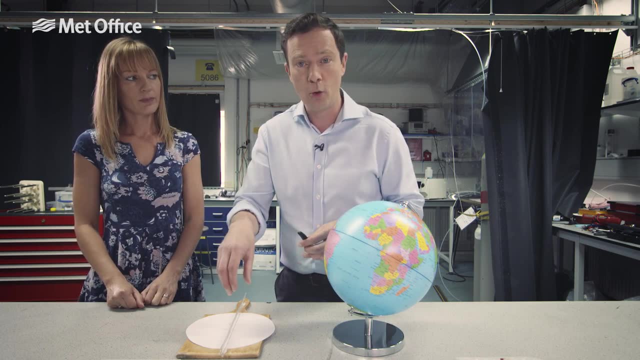 a ruler and a pen. I'm also going to need a little bit of assistance. so Helen is joining me and she's going to spin the disc of paper as if it was the earth, as if we were looking down from the north pole, from above the north pole. That means you need to rotate that disc anti-clockwise. I'm going to. 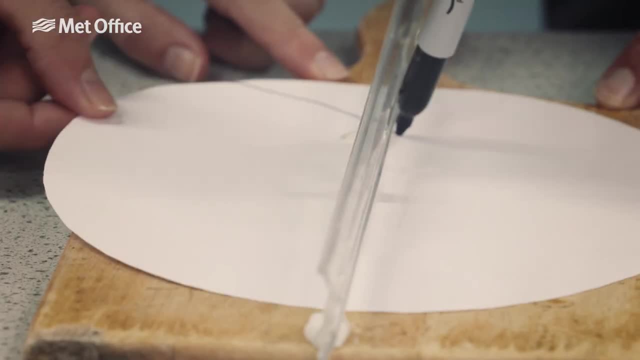 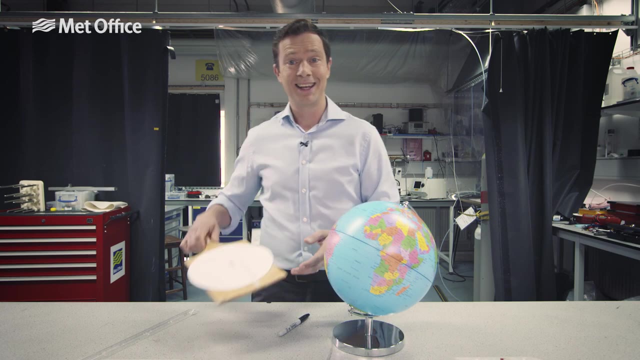 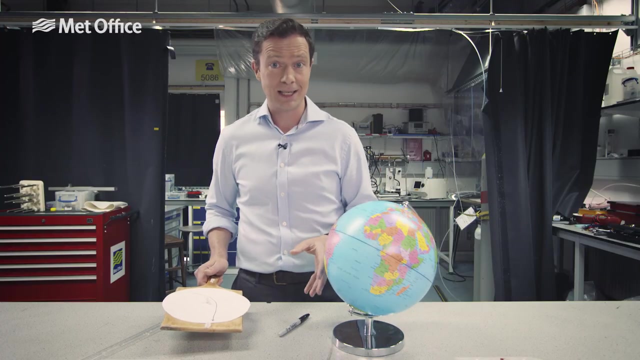 draw a straight line along the ruler as Helen rotates that and just look what happens. The spin of the earth means that that straight line is not straight. If you were looking from here, you'd see that the winds will be bending round to the right. That is Coriolis in action in the northern hemisphere. 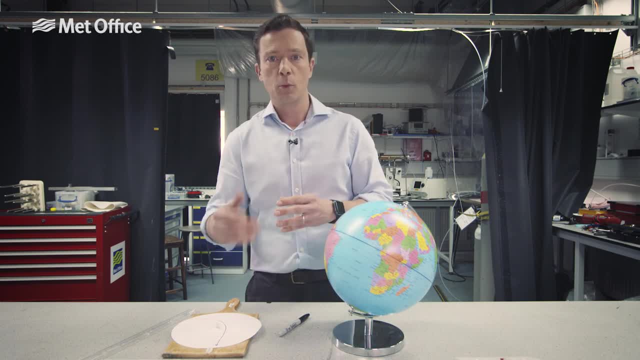 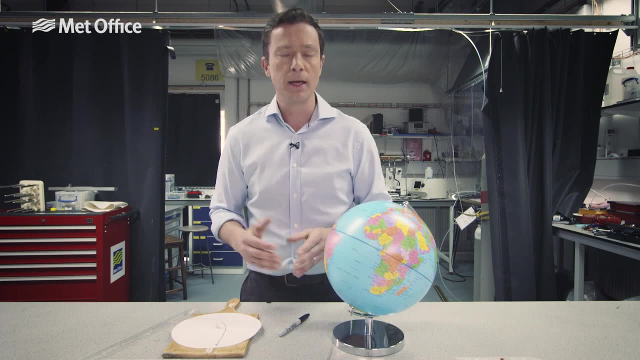 If it was the southern hemisphere, we were looking from below the south pole- we would spin the disc the other way, clockwise. Try that at home and you will see that the winds bend the other way to the left. Now you may have heard that Coriolis makes the water spin down plug holes. 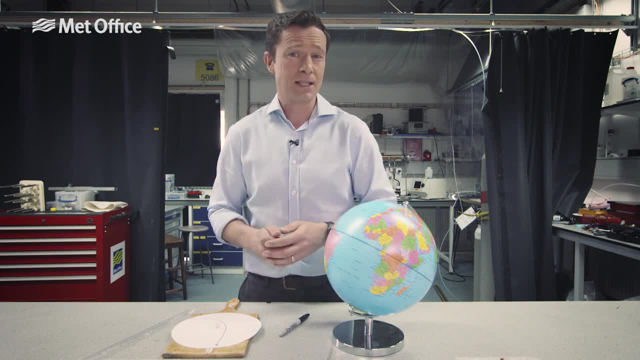 in different directions in different hemispheres. That turns out to actually be a bit of a myth. Plug holes are just too small a scale for Coriolis to really have any impact, But it is the reason why low pressure systems and tropical storms rotate anti-clockwise in the northern hemisphere.